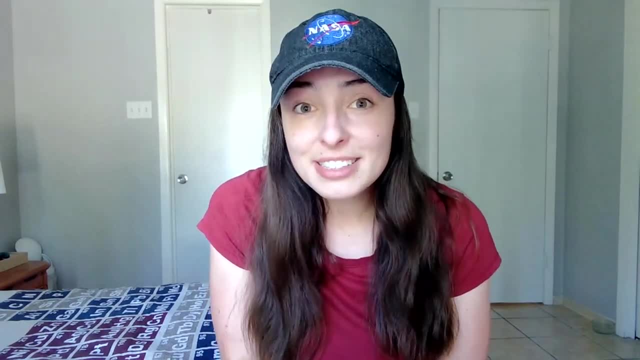 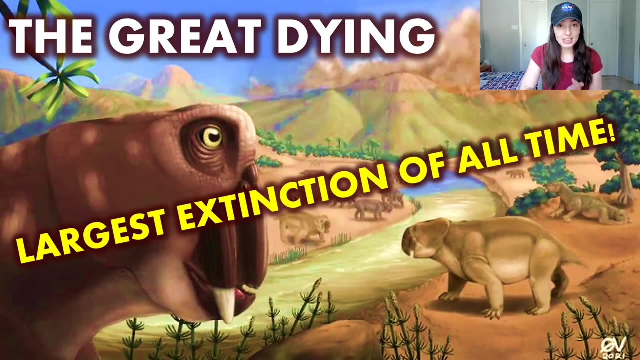 Ever wonder what really happened that led to nearly 96% of all species on Earth going extinct at the end of the Paleozoic era? Well, in today's video I'm going to be talking about the Great Dying, or the largest extinction event of all time. This is one of the big five recognized. 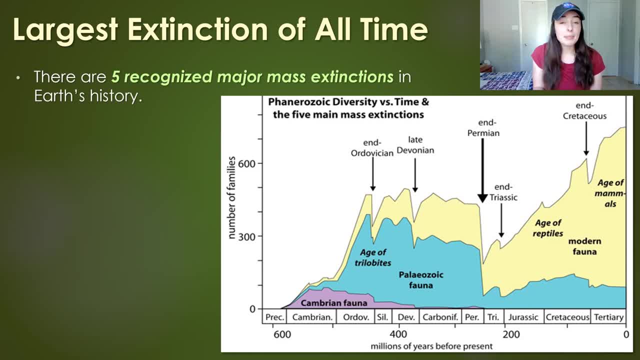 major mass extinctions throughout Earth's history and it happened at the end of the Permian period, which is the last period in the Paleozoic era. We can see on this big diversity chart here that the five big dips, or the late Ordovician, late Devonian, end Permian, which is the one we're. 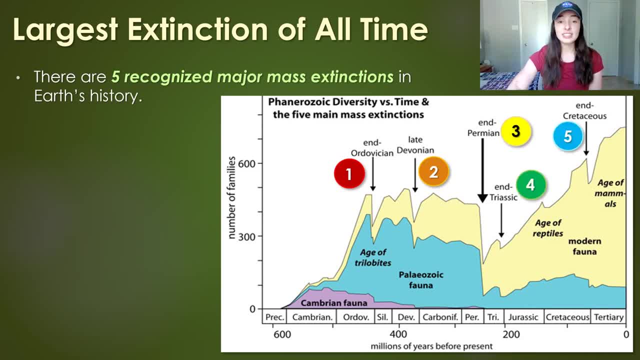 talking about today: end Triassic and end Cretaceous extinctions are all plotted here throughout Earth's history. Number three here: the end Permian was the largest extinction event of all time. However many times people incorrectly state that nearly 96% of all life on Earth. 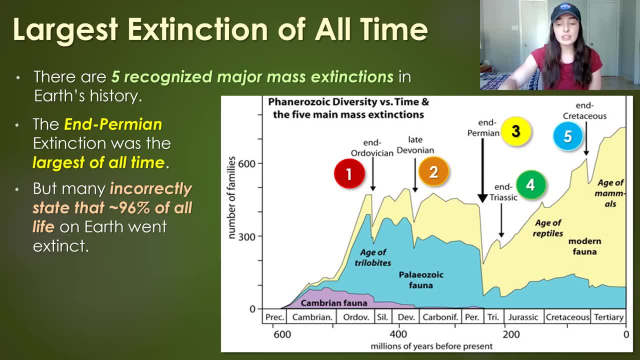 went extinct due to this end Permian extinction event. That is actually incorrect because that percentage actually includes the devastation from an earlier extinction event earlier in the Permian period called the end Guadalupean extinction event. Just to show you where we're at in the 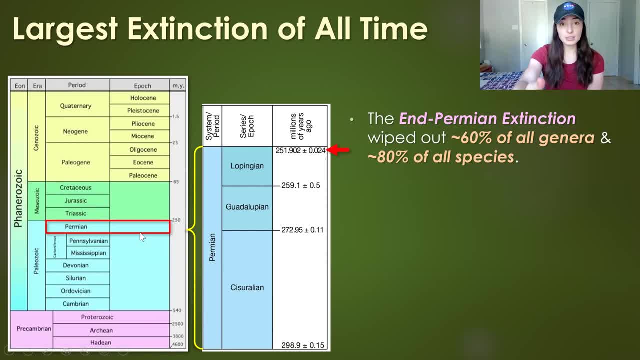 timeline here. the Permian period was the last period in the Paleozoic era, as shown on this timescale, going from oldest to youngest, from bottom to top, and it goes from around 299 to 251 million years ago, 60% of all genera and 80% of all species were wiped out, which is still the 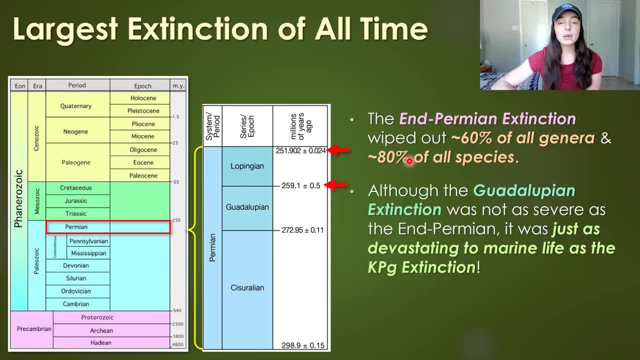 largest extinction event ever. so it's still pretty devastating, But the Guadalupean extinction, which occurred right at the end of the Guadalupean series or epoch within the Permian marine life, was hit just as hard as it was during the KPG or Cretaceous-Paleogene extinction that wiped out. 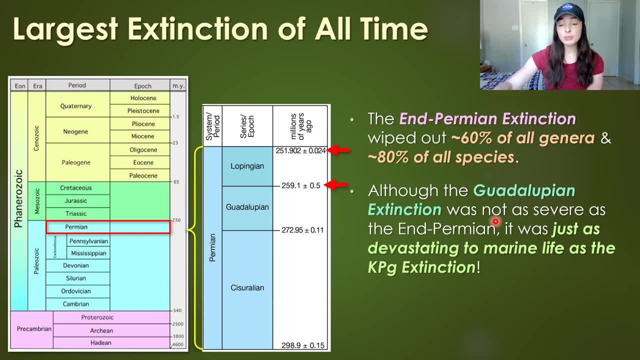 the dinosaurs, And although it wasn't as severe as the end Permian, it was still a very, very extinction. Many people argue that it should be included in the big major extinction events, of which we have five currently, so it would be the sixth one, unless you count today as the sixth. 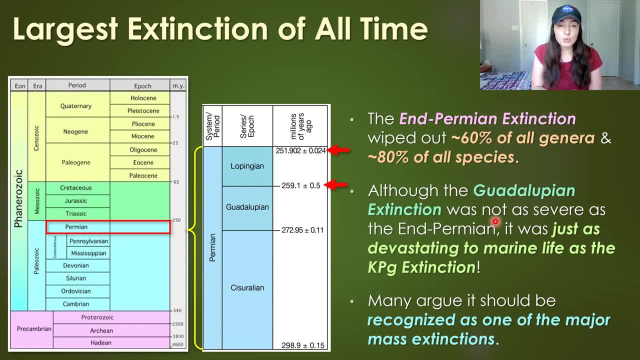 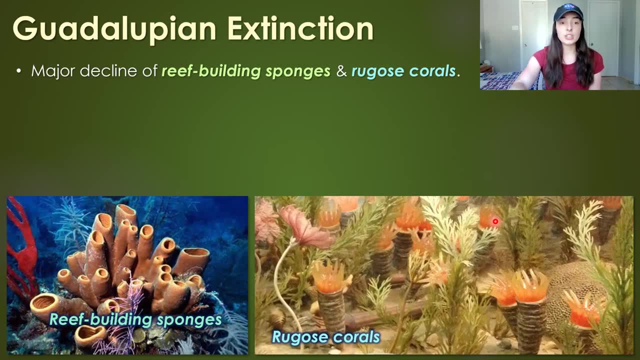 one, so maybe the seventh, But anyway it should be included, probably. So we'll talk about the Guadalupean extinction event first and then we'll get into the end: Permian great dying extinction event. This extinction event marked a major decline of reef-building sponges and rugose corals. 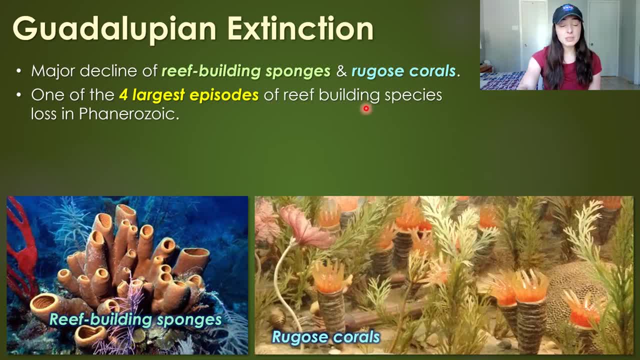 and this event was actually one of the most important events in the history of the Guadalupean history. It was one of the four largest episodes of species loss amongst reef builders in the Phanerozoic, which includes the Paleozoic, Mesozoic and Cenozoic eras, aka around 500 million years ago. 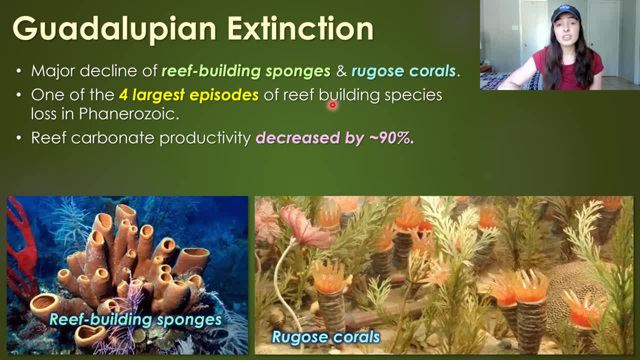 to present, And during this event, reef carbonate productivity decreased by 90%. So the production of carbonate by reef builders decreased by 90%, And recovery of reefs, which are ecologically essential organisms and communities, took nearly five to seven million years, only to then be decimated again at the Permo-Triassic. 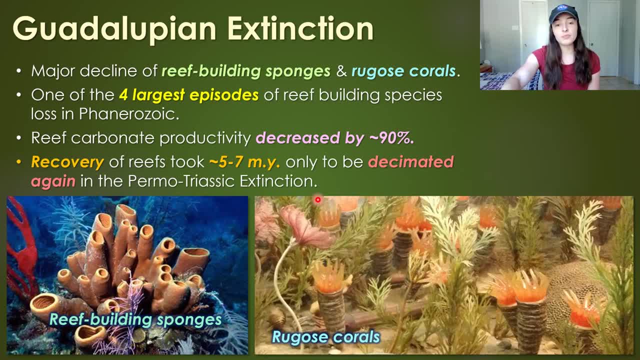 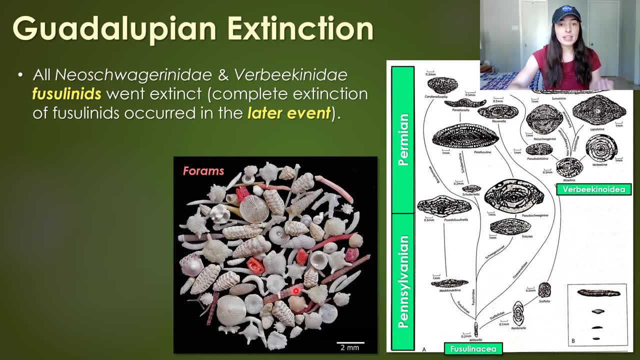 extinction or the late or end Permian extinction. Forams, or foraminifera, were also hit hard during this period, and these are also carbonate-precipitating organisms. although they're microorganisms, They're not as macro as coral reefs, but they're still very important ecologically and produce a lot of carbonate, And one of the things that we're going to talk about today is the carbonate-precipitating organisms, or the late or end Permian extinction, And one of the things that we're going to talk about today is the. 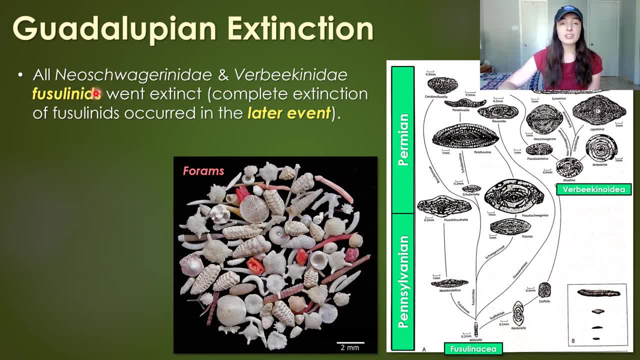 type of forum called Fusilinids, which were crazy abundant during the late Paleozoic, went nearly extinct during the Guadalupian extinction. All of their later larger, more complex forms, like the families Neoshrongerinidae or Veribukinins went extinct. 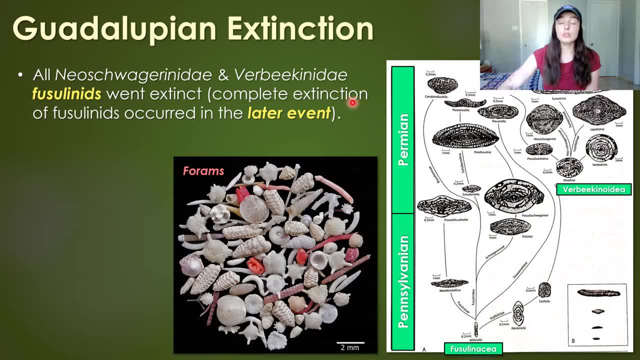 due to this extinction event and then the complete extinction of Fusilinids occurred in the later end, Permian extinction, Only smaller and morphologically simpler forms of forams survived, And so the later and more complex forms of forams like the Neoshrongerinidae. 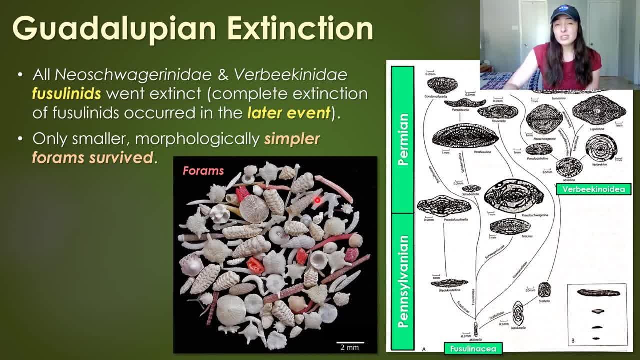 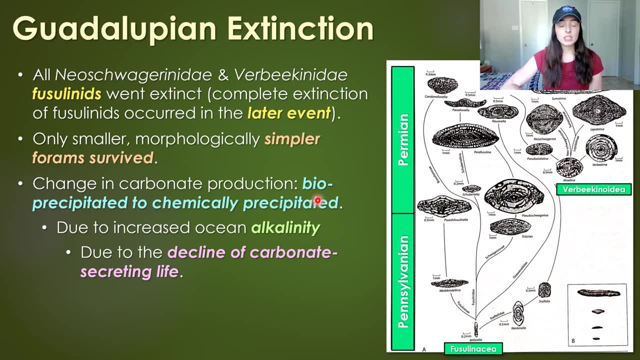 survived this Guadalupian extinction and the initial decline of Fusilinids at this extinction event probably made their extinction more likely during the later extinction event. Overall, with all the effects the Guadalupian extinction event had on carbonate-precipitating organisms there, 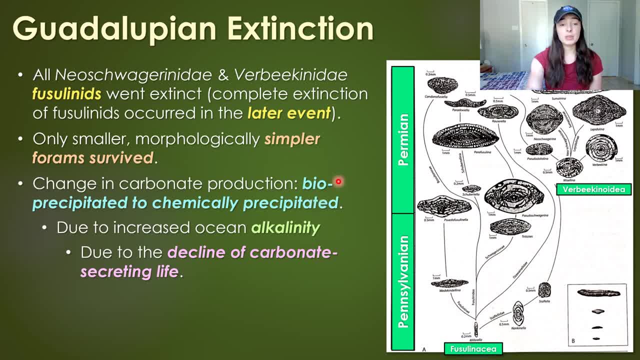 was a fundamental change in carbonate production, That is, it went from being mainly bioprecipitated or biologically induced mineralization to chemically precipitated or abiotically produced, which was due to a decline of carbonate-precipitating organisms. There was also declines of 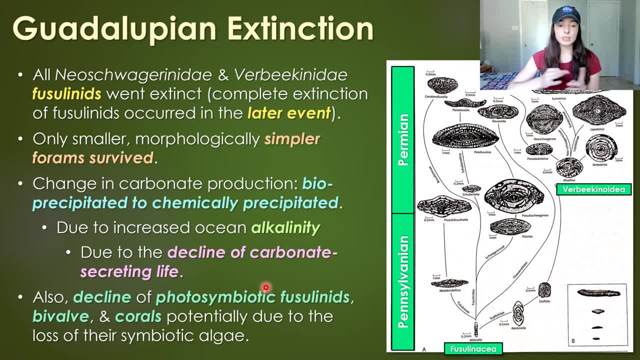 photosymbiotic Fusilinids, bivalves or clams and corals, potentially due to loss of their symbiotic algae. like the bleaching of corals today, That's due to the loss of their algae because of the changing environment, so that could have potentially been the reason for the 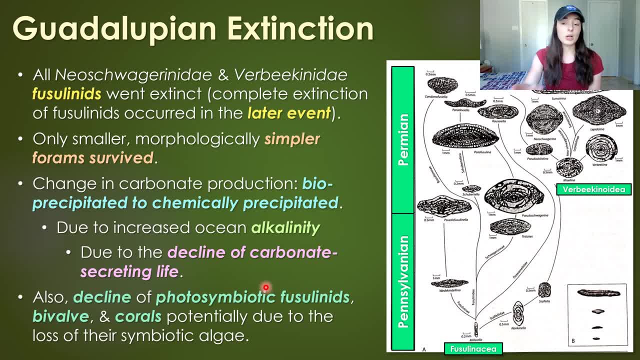 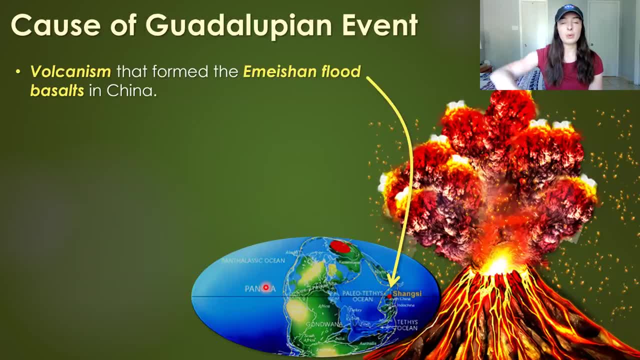 decline of the photosymbiotic species at this time as well. In any case, the Guadalupian extinction event was much harder on marine life than it was on terrestrial life. But what caused the Guadalupian event to begin with? It's likely that volcanism caused this event, specifically the 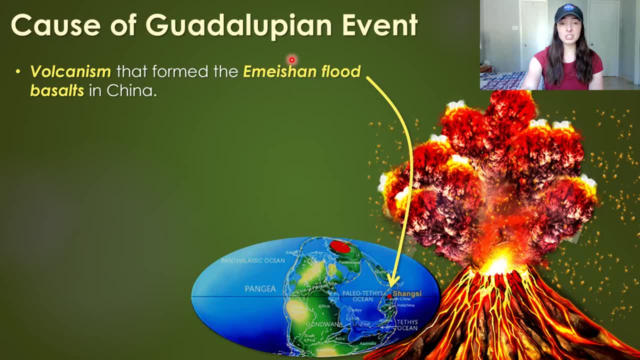 volcanic eruptions that formed the Emishan flood deposits in China. I don't know if I'm pronouncing that right. sorry if I'm not. In any case, these lava flows initially covered an area of over a million square kilometers, and we can see the little red dot here that shows those. 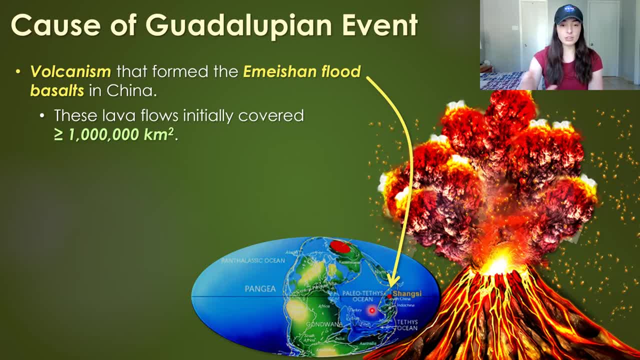 deposits in the map of the continental formation that would have been occurring at that time, And we can also see the signature of volcanism in ocean sediments at the time, which show elevated mercury, which is a signature of volcanism, And then we also see a negative carbon isotope. 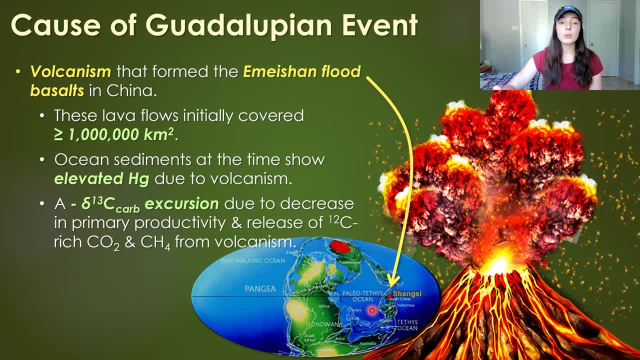 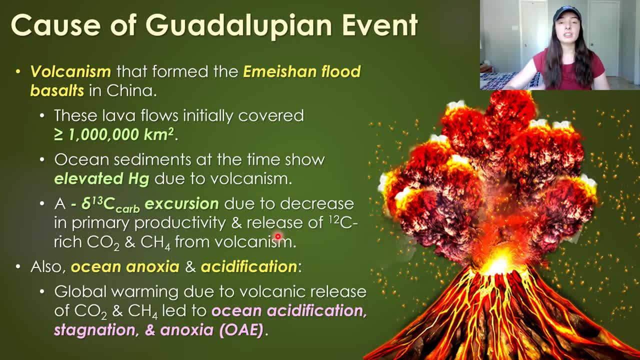 excursion due to a decrease in primary productivity and also the release of isotopically light carbon from the volcanoes. But volcanism alone didn't cause the extinctions. it caused what started the extinctions, That is, global warming, ocean anoxia or the lack of oxygen in the ocean. 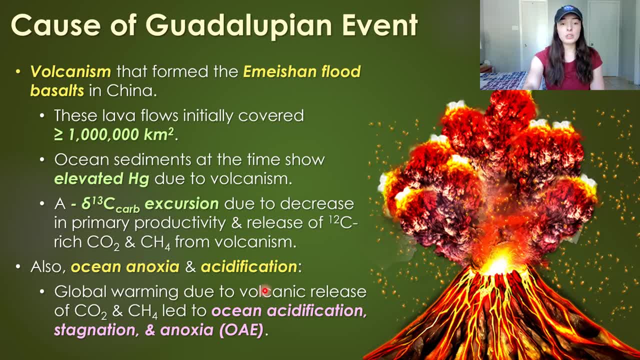 and ocean acidification. Global warming due to the volcanic release of CO2 and methane led to the ocean acidification, stagnation and anoxia in what's called an OAE or an ocean anoxic event, And the lack of oxygen caused a lot of deaths among marine animals, which is why this event. 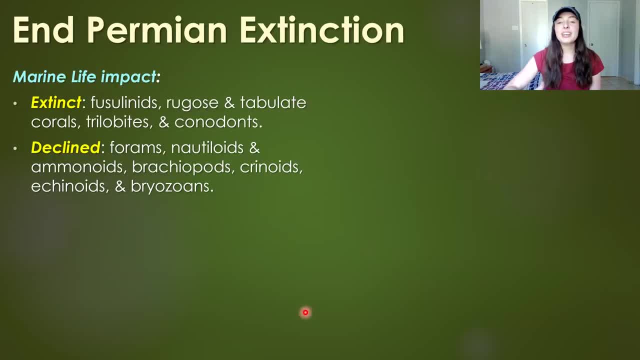 hit marine life harder than land life. But now getting to the end-Permian extinction event, the great dying, the largest extinction of all time. This extinction event affected both marine life and terrestrial life, but we'll start with the marine effects first. 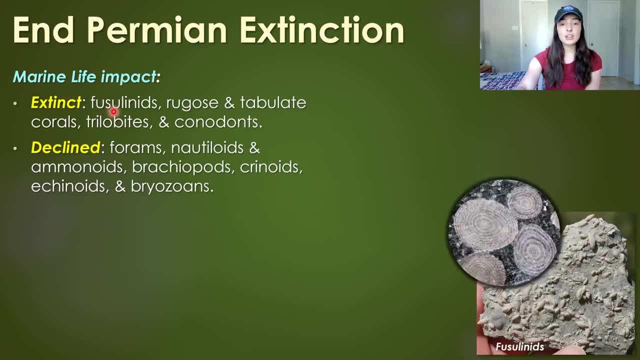 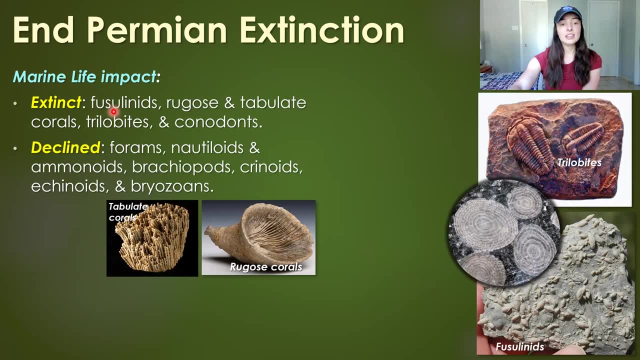 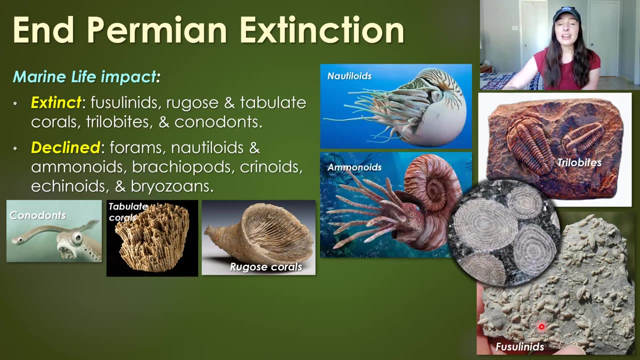 The marine life that was affected included the extinction of fuselinids, rugose and tabulate corals, trilobites, which dominated Paleozoic seas, and conodonts, And it caused the decline of forams other than fuselinids and nautiloids and aminoids- brachiopods. 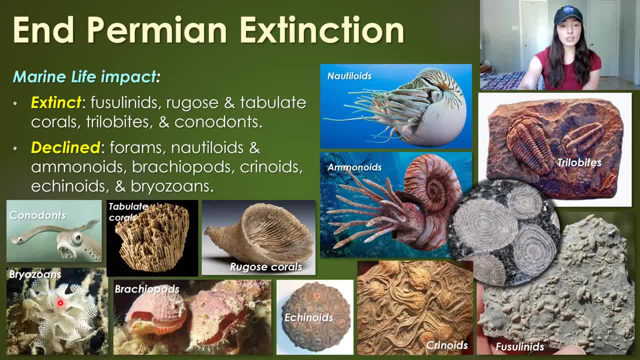 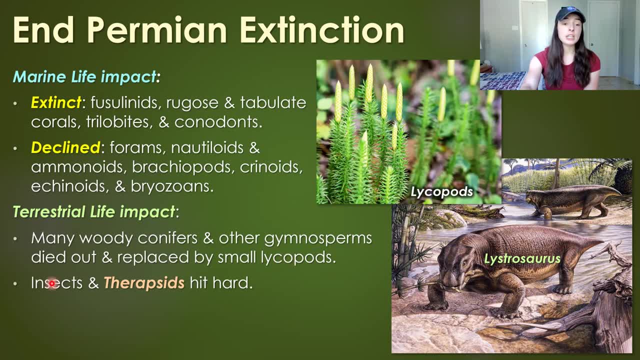 crinoids, econoids and bryozoans, But terrestrial life, like I mentioned, was also impacted. For example, many woody conifers and other gymnosperms died out and were replaced by small lycopods- I talk about lycopods in my Ice Age and Giant Insects. video about the Carboniferous. 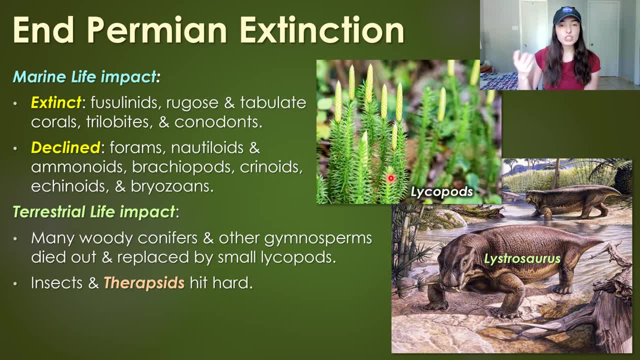 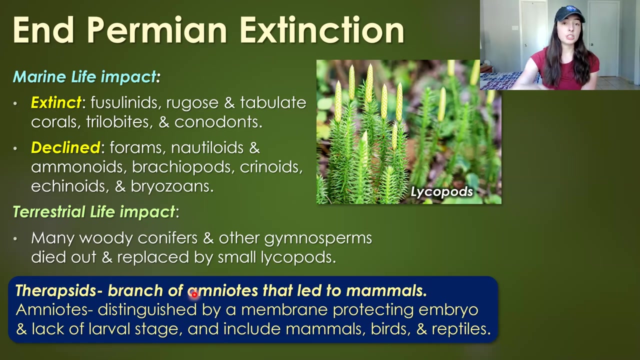 and how they got huge in the Carboniferous, like 100-foot tall lycopod trees that covered swampy areas and then died and accumulated to make the vast coal deposits. Other than plants, insects and therapsids were also hit very hard. Just to recap, therapsids are a 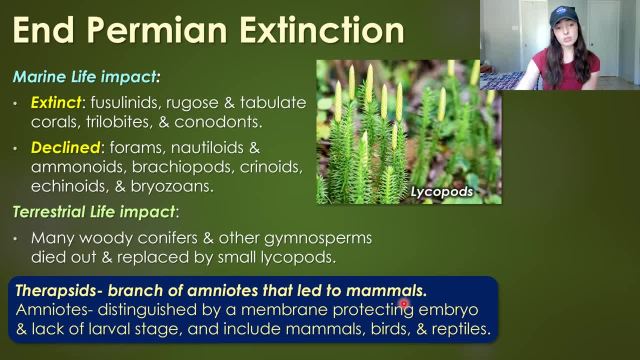 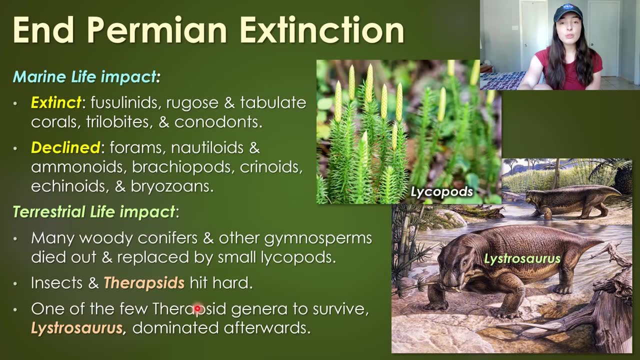 branch of amniotes that lead to mammals, And amniotes which evolved from amphibians in the Carboniferous are distinguished by the fact that they can be found in a variety of species, including mammals, birds and reptiles, One of the few therapsid genera to survive this extinction event. 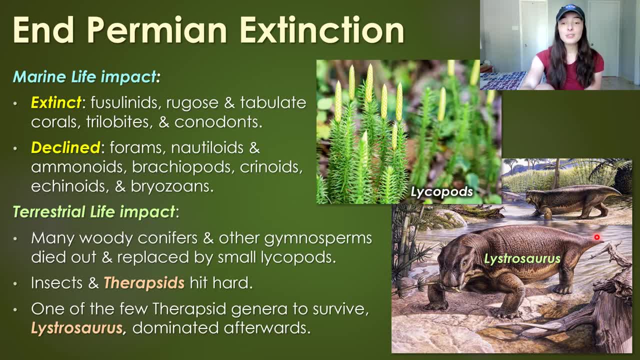 was Lystrosaurus- I hope I'm saying that right And we can see a picture of this guy here as well as in the thumbnail for this video- And they grew to dominate after this extinction event, because after an extinction event the environments and ecological niches are pretty much cleared out. 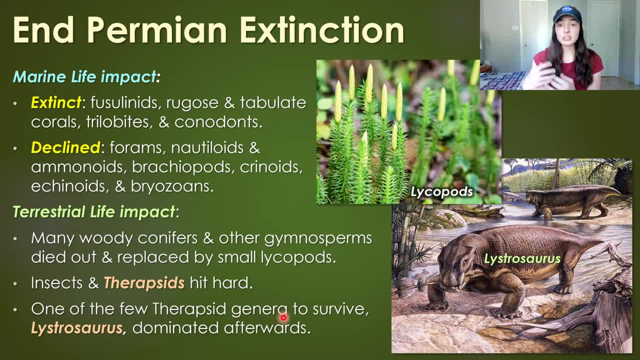 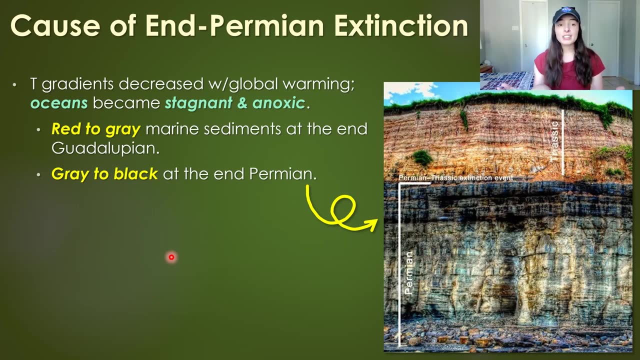 And whatever survived can radiate because there's nothing to compete with or run away from. So now that we know the effects of the Empyrean extinction were so drastic, we're probably wondering what caused this extinction event in the first place. Was there an asteroid impact? 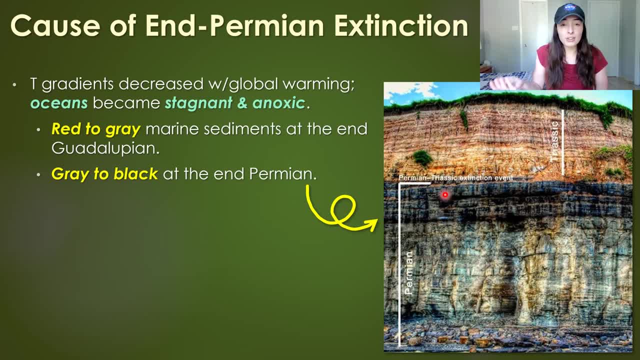 What happened? Well, there was no asteroid impact to set off climate change that caused an extinction event like at the end of the Cretaceous. Instead, what happened was temperature gradients from equator to poles decreased with increased global warming, causing oceans to become stagnant and 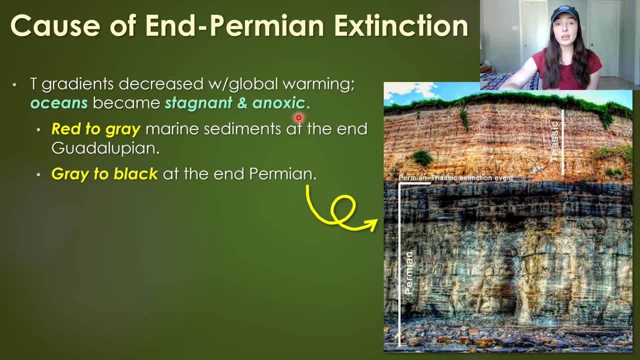 anoxic. The reason temperature gradients are important is because they greatly affect ocean circulation, because strong temperature gradients from equator to poles mean strong winds and mean strong surface ocean circulation and upwelling and mixing of the ocean and well-oxygenated oceans. 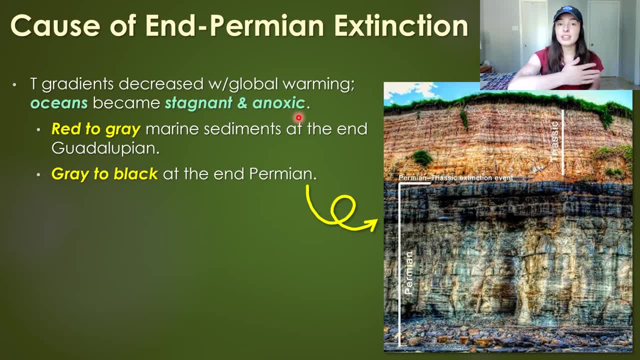 whereas weak temperature gradients cause the opposite and eventually lead to stagnant and anoxic oceans that aren't well-mixed, And so we're going to have to figure out how we're going to do this. We can see this in the rock record, with a switch from red to gray marine sediments at the 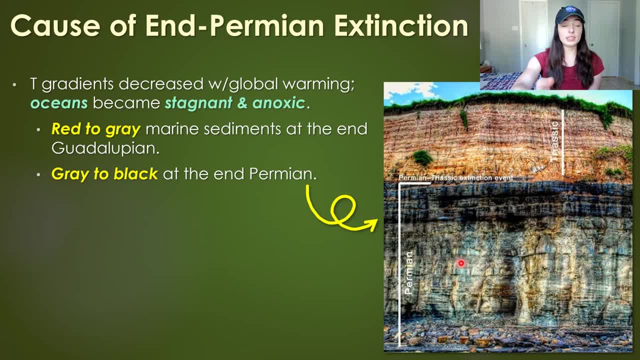 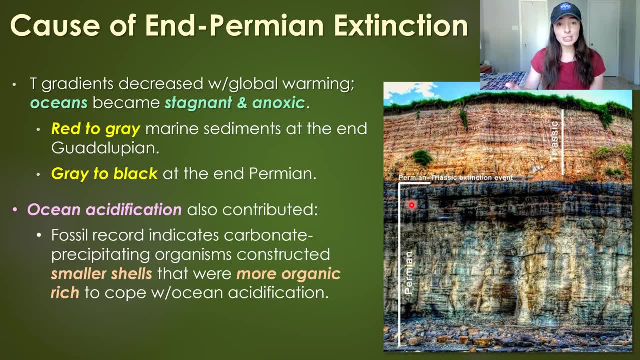 end of the Guadalupian, which marks the end Guadalupian extinction, and then a switch from the gray to pretty much pitch black at the end of the Permian Ocean. acidification, just like with the end, Guadalupian extinction also played a major role. In fact the fossil record indicates. 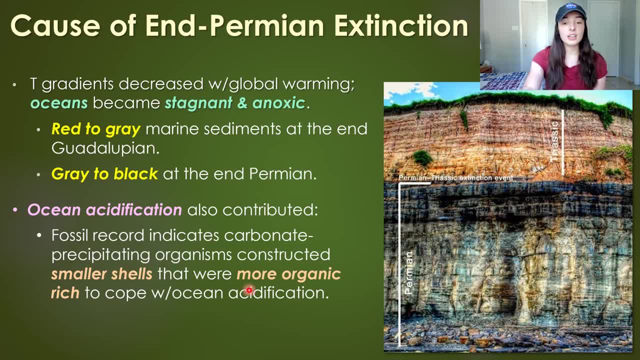 that carbon precipitating organisms constructed smaller shells that were more organic rich to deal with the ocean acidification during this time. In short, carbonic precipitation is favored in alkaline conditions and not acidic ones, and the acidification of the ocean would mean that. 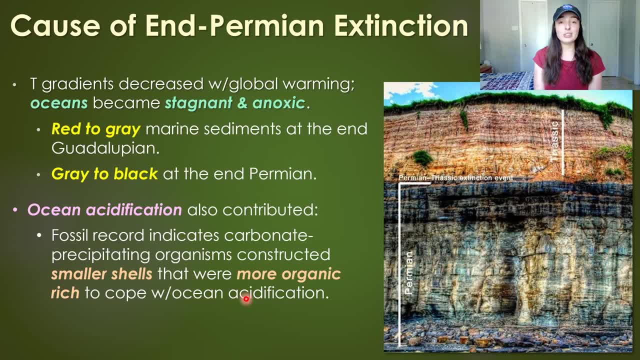 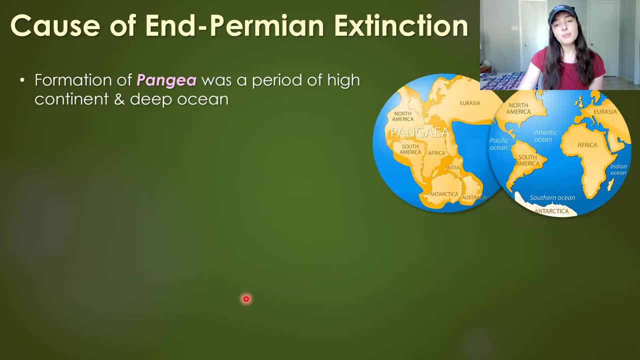 carbonic precipitation is less favorable for the biological organisms that secrete it to create their skeletons or shells, and so they would have incorporated more organic matter, less carbonate, to account for this acidification, and also would have made smaller shells and skeletons. The formation of Pangea. however, 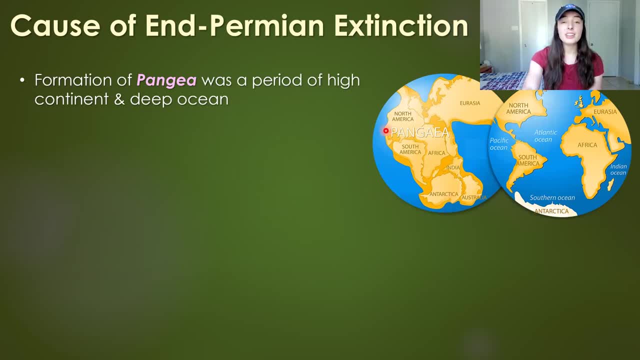 is not to be forgotten. During this time, Gondwanaland had collided with the northern continental masses to become Pangea, one massive supercontinent which was actually pretty high in terms of elevation, whereas the one big ocean at the time was pretty deep. This changed both. 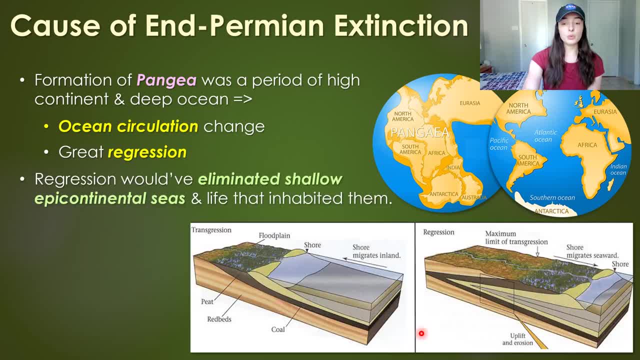 ocean circulation and caused a great regression. Regression, or the lowering of sea level causing the movement of the basin margin, basin word or sea word would have eliminated the Pangea and the two epicontinental seas which hosted a lot of life during any time that they've. 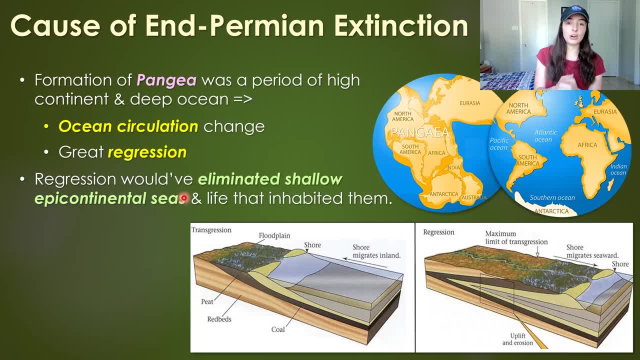 existed on continents and all the life that inhabited them would have also become eliminated. The changes in ocean circulation would have also exacerbated the ocean stagnation and anoxia, further exacerbating the extinctions occurring to marine life. But just like with the end Guadalupan. 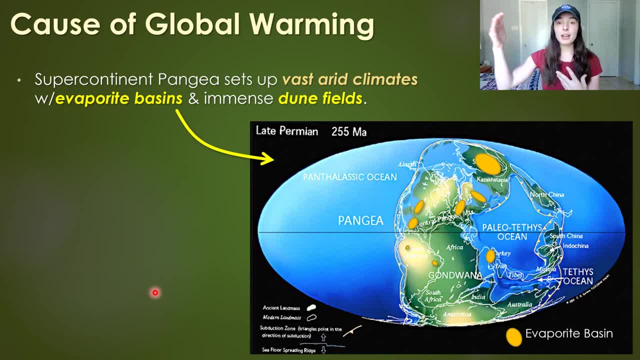 extinction, there had to have been a cause for the second spike in global warming that then caused the and acidification, etc. Formation of Pangea not only contributed to a loss of epicontinental seas and changes in ocean circulation, but also set up vast arid climates with evaporate basins and. 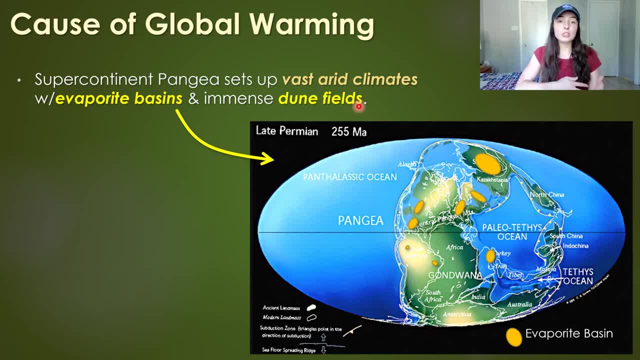 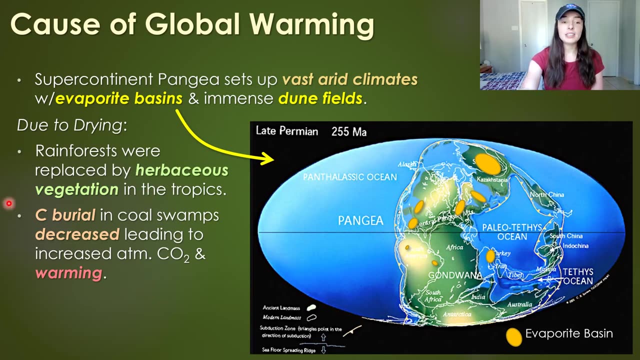 immense dune fields. If you know anything about the Carboniferous, which is the period just before the Permian period, this was a very swampy, moist time, with wetlands and tropical forests And, because of the drying rainforests were replaced by herbaceous vegetation in the tropics. 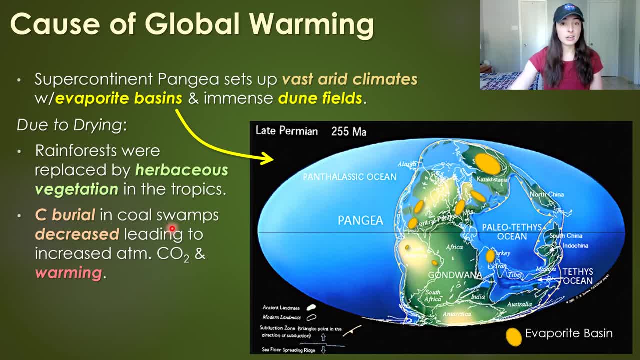 and carbon burial in coal swamps, which characterized the Carboniferous period, decreased drastically, leading to an increase in CO2 and global warming due to increasing greenhouse gas effect. This global warming would have then been exacerbated by the melting of methane hydrates and the release of that methane to the atmosphere, because methane is just like 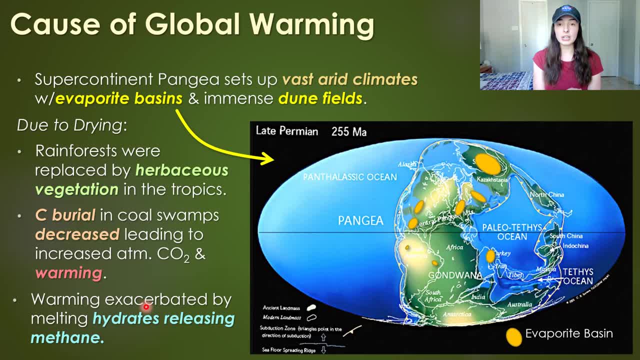 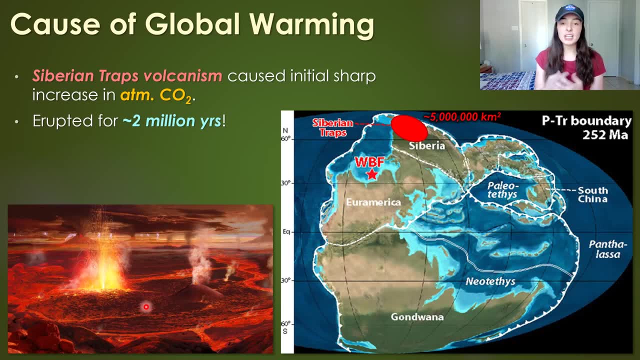 carbon. In fact, it's a much more powerful greenhouse gas than carbon dioxide. But the real cause that really just set off the end Permian extinction event and all of these climatic changes that were associated with it was the eruptions of the Siberian Traps. 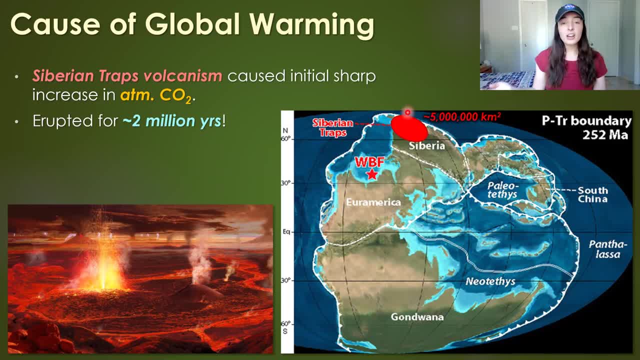 These volcanic eruptions are estimated to have caused lava flows that covered an area of over 5 million square kilometers, and I've seen estimates of 7 or 8 or more, So I don't know exactly the estimate, but that's a lot, And it was much larger than the around 1 million square. 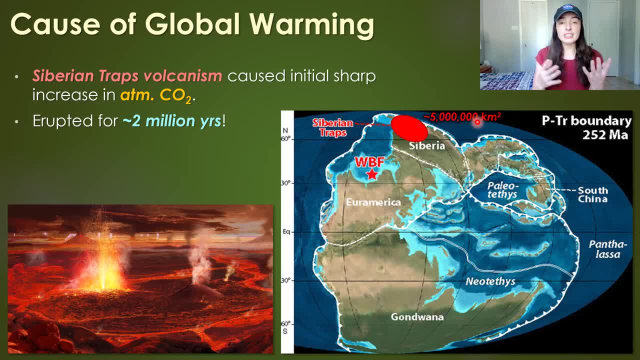 kilometer lava flows of the end Guadalupeans. So it was an even larger event, which is why, eventually, the extinction event was even more drastic, in association with a symphony of climatic disasters and the formation of Pangea and ocean circulation change and all of these things. 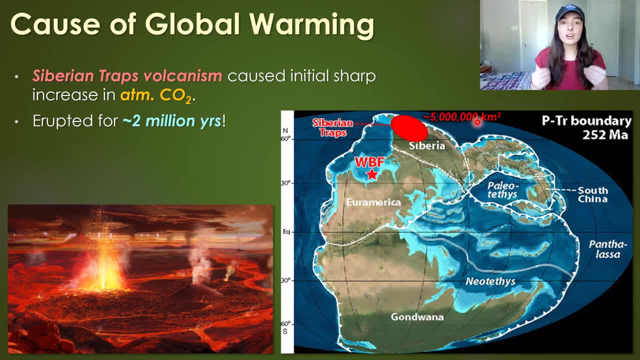 that came together, But this was really like the initial cause of the warming, because all of this volcanic event was a result of the eruption of the Siberian Traps, So it was an even larger event, which erupted for 2 million years, caused a sharp increase in atmospheric CO2, because that's what